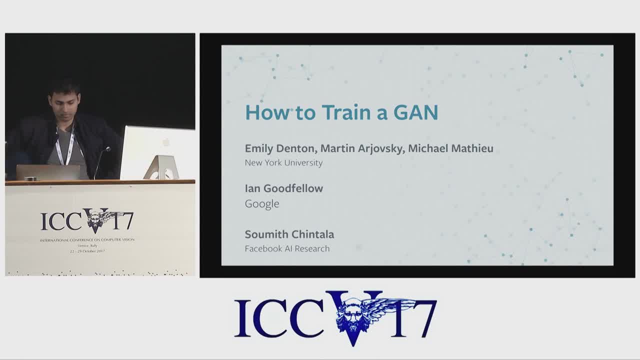 tricks that are necessary to make them really work. Hello, So, as Ian said, I've done a lot of empirical work on GANs and this talk is just giving a lot of tricks that we learned over the years on how to train GANs, like what tricks you need to use As a heads up. this talk doesn't. 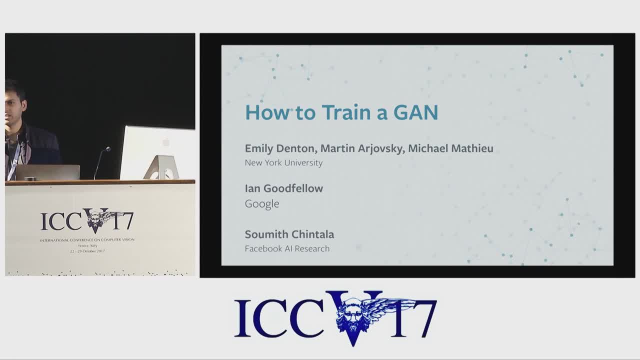 really cover GANs, but it does give you a little bit of an idea of how to train GANs. So if you have any like, any theory or any like, some of these tricks are very arbitrary, like someone just came up with, like, oh, I want to try this and it seems to work in this setting. So these 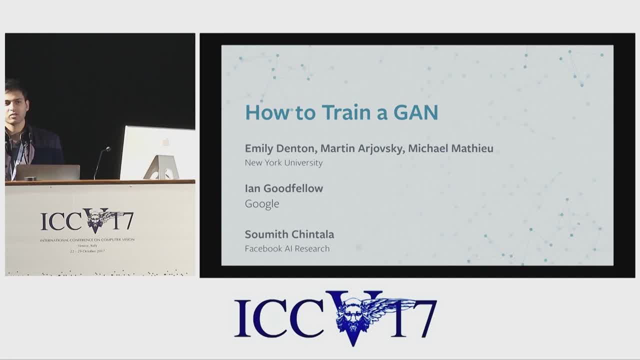 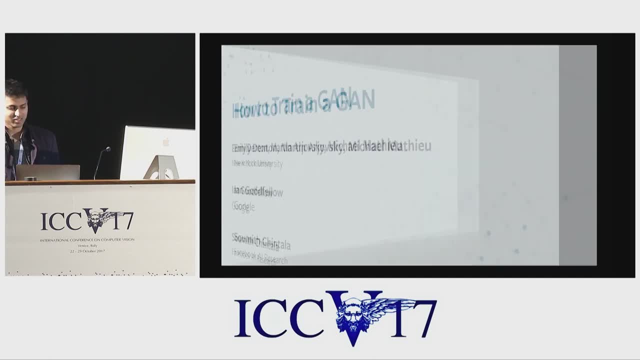 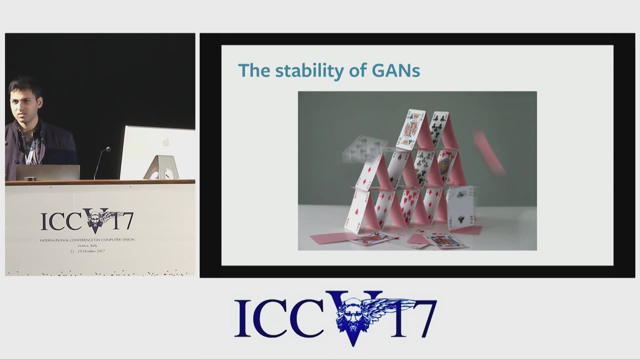 tricks. take them as hints rather than a hard line. oh, this is a peer-reviewed idea. So a little bit about GANs that Ian mentioned in his talk. GANs are not considered stable to train. They're very- finicky. So if you go to GitHub, find someone's GAN implementation, try it on your data set. 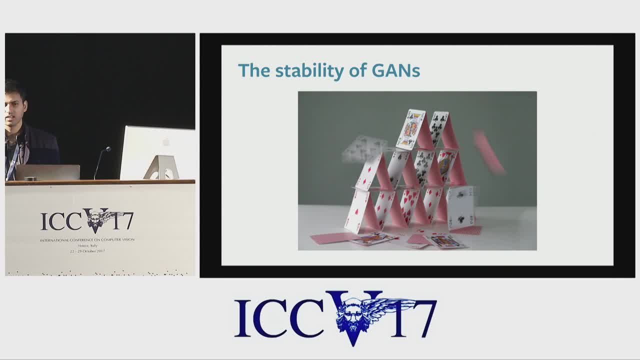 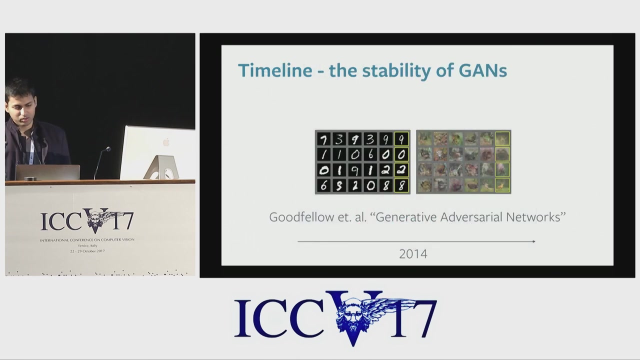 there's a very good chance that nothing will come out of it. So they're not like con nets for classification, where you just take a con net, you put it on your data set and suddenly accuracy improves a lot. So a little bit about the timeline of GANs. 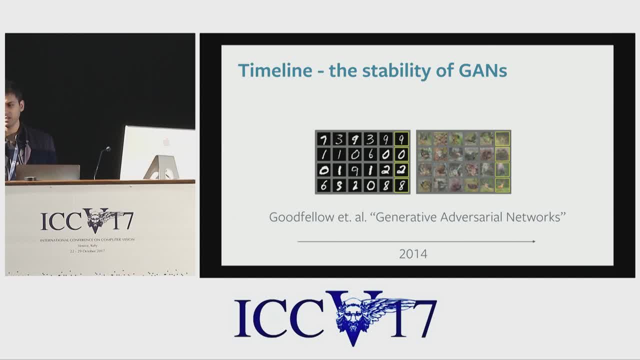 Ian introduced GANs in his paper in 2014, and he showcased samples on MNIST digits and on CIFAR, And his initial paper covered the concept of GANs, but it was on very small-scale data sets And we tried to replicate it on larger. 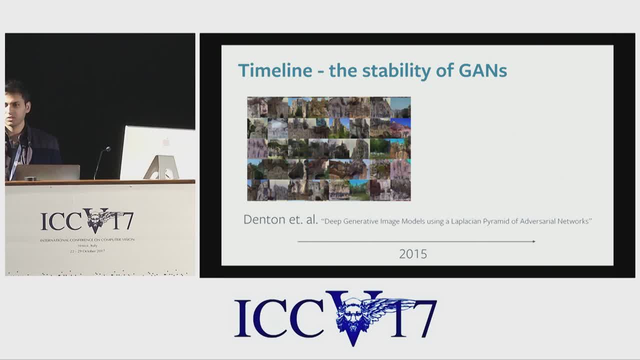 data sets. His initial images were also 32 by 32 pixels in size, So we tried to scale it up in our subsequent work to 64 and 128 pixels, And as we were doing this, we had to do a lot of things that we're not super proud of. 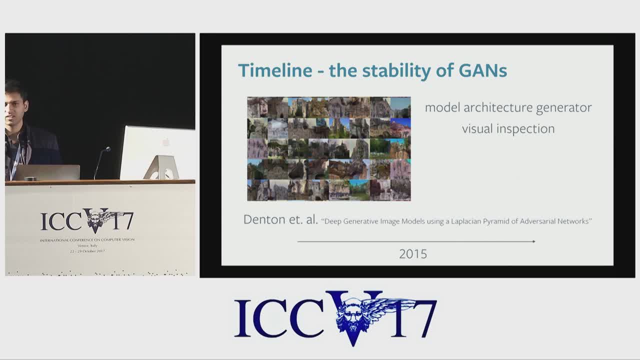 We had a model architecture generator that would just generate random con net architectures and then train them and see which model seems to be stable. We had to do a lot of visual inspection because, as Ian mentioned in his talk and as Mihail mentioned as well- and I think many 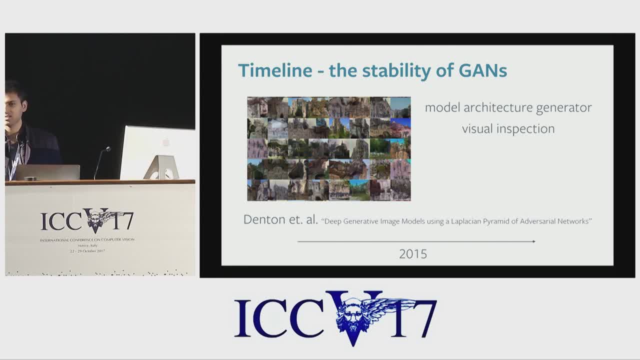 other people will talk about it. evaluating GANs is a hard, hard problem. in general, Visual inspection is only a hack of sorts, As Mihail showed. even if the samples look visually like they don't have any mode, collapse and stuff they still might. And we did a lot of hacks. We tried a lot of hacks like 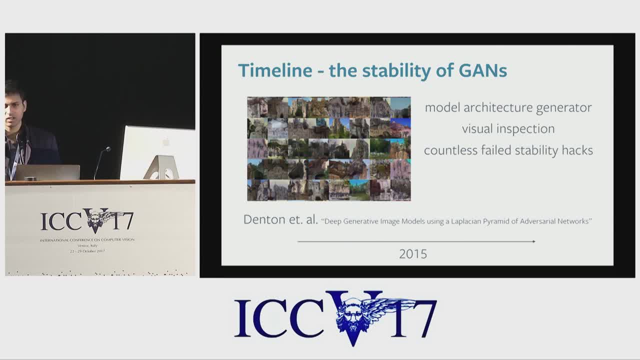 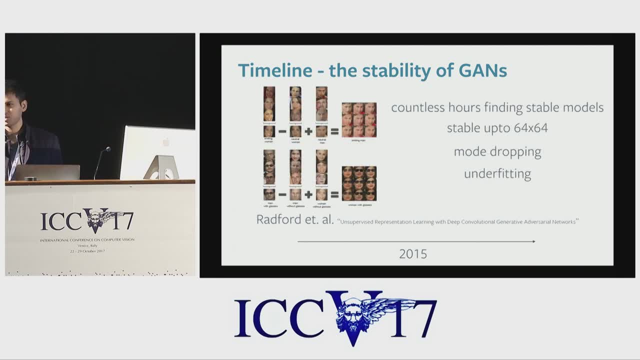 trying to balance the generator and the discriminator so that the training is more stable And, like I think, partly it was just our hyper parameters worked out. So we published the paper And then Alec Watford, in 2015, pioneered DC GANs. They were the stable architecture that 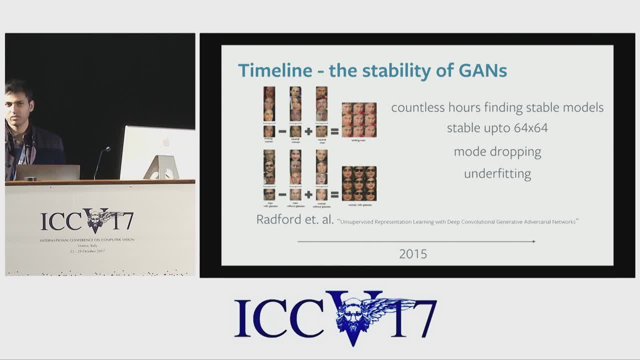 seems to work for image generation, largely regardless of what you threw at them, And there's a lot of fun experiments people have done with DC GANs, just showcasing how stable they are. are people through data sets like manga generation and handwriting generation and all? 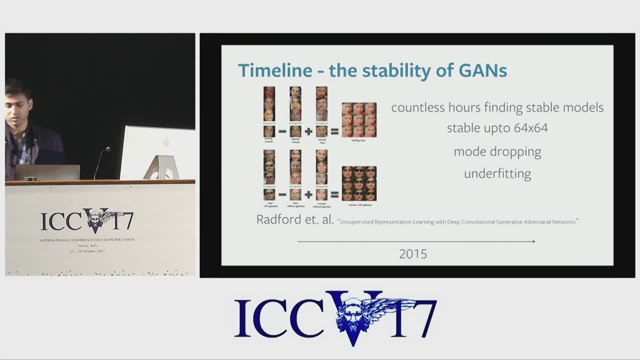 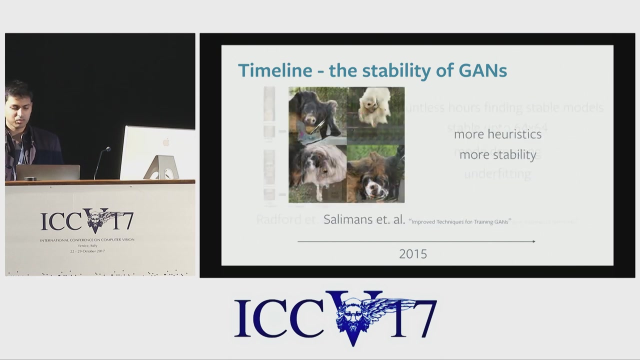 of these various different kinds And they seem to work fairly well. But DC GANs have this problem of mode dropping, where they would only capture certain parts of your distribution rather than generating an overall scheme of things. And then people try to find more heuristics, more stability. 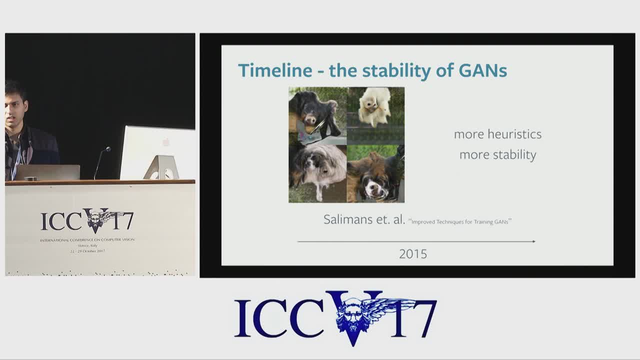 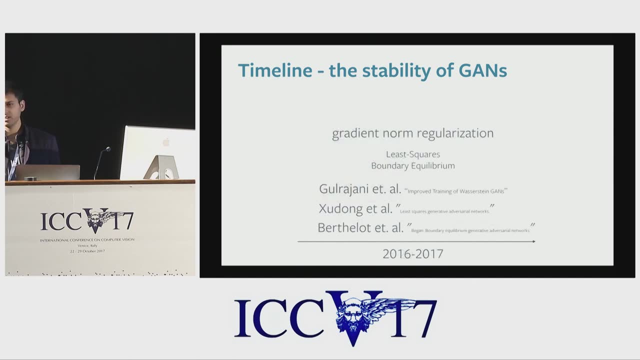 Tim Salomons and team from OpenAI published this improved training of GANs And they had four or five tricks in there that generally seemed to improve the stability of training GANs, And 2016 and 2017 saw an explosion. 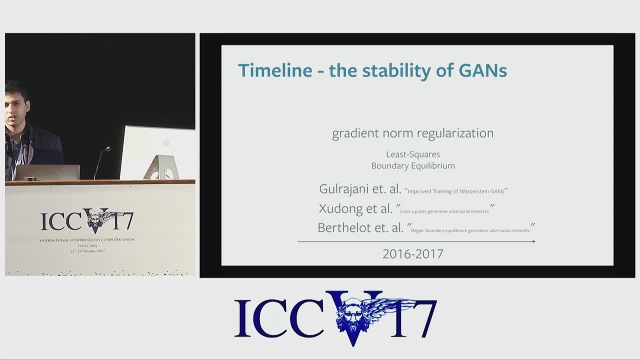 of papers, And one of the big ones that came from three or four different papers. it's like three or four people, sets of researchers separately approached the problem of how to stabilize GANs, And one of the common things they came up with is: 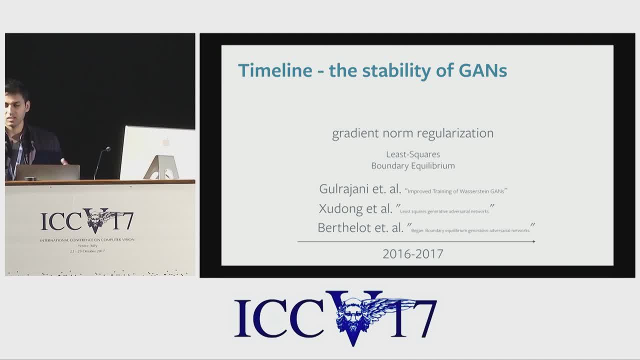 let's stabilize the norm of the gradients And that seems to be working pretty well, And there's also been some other formulations that are stable on like they're better on some data sets. Boundary equilibrium GANs was one of the recent ones. 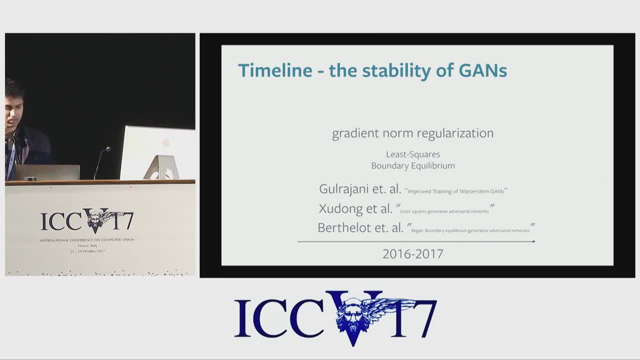 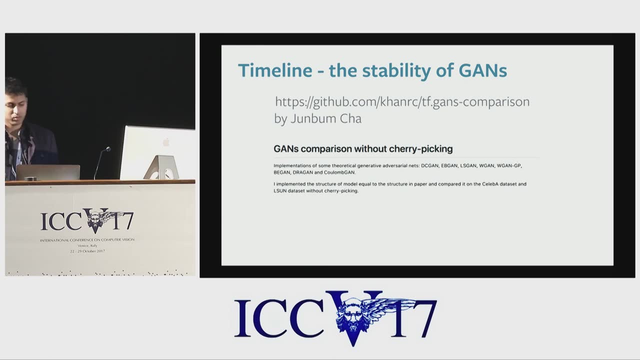 that try to get like an SVM style tinge to it And one of the interesting projects I saw recently. quickly read through the GitHub- read me, but there's this implementation by this person called, who. I don't know if you've heard of him, but he's like. 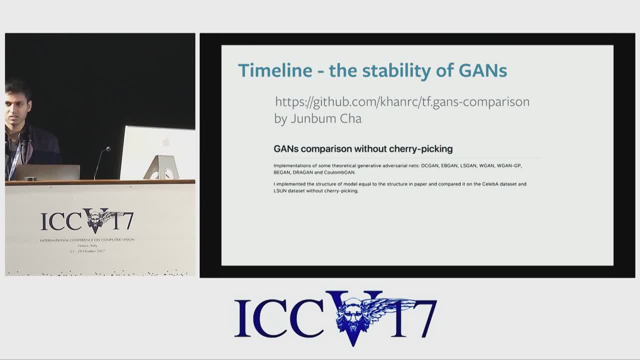 he independently just took implementations of GANs And without cherry picking, he just ran two data sets through all of these different variants of GANs and then stopped at some particular iteration on all of them and saw what samples were good or not. 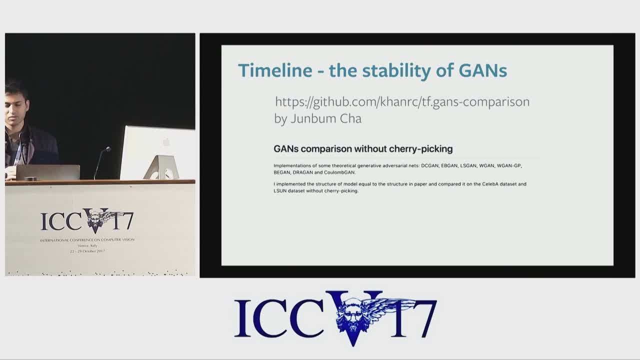 And it's interesting because each of these papers separately. when the authors are trying to publish the papers, they do cherry pick to an extent, and I'm no exception. So it was just interesting to see someone take all of these implementations And they reported, for example, on something: 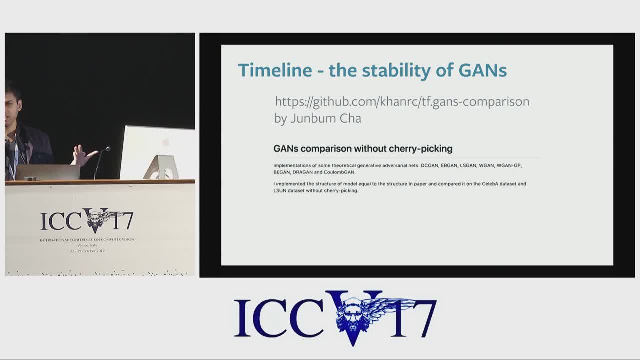 like a big and boundary equilibrium GAN. They're like, oh, this works really well on this data set, But then if on this other data set it completely does not work, And to an extent I'm sure there are subtle things. 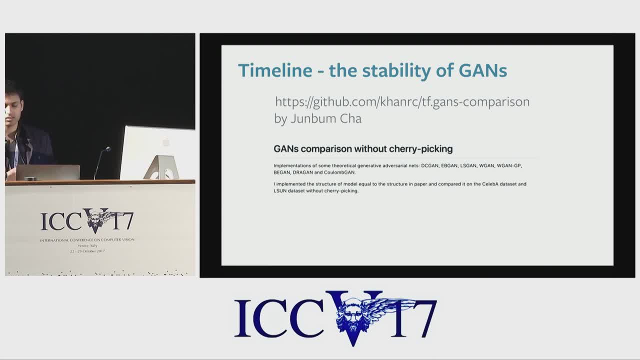 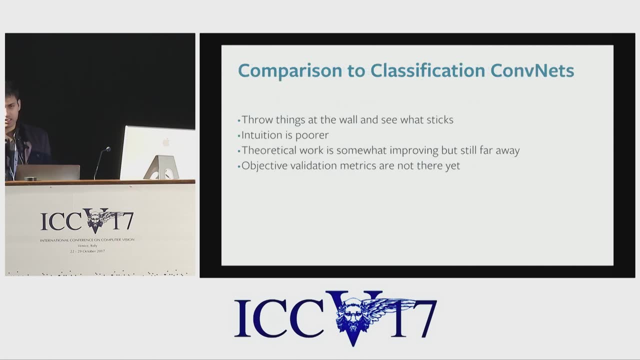 in this particular person's implementation, But I thought it was generally interesting from an empirical standpoint if I had to implement some idea like how it might or might not turn out. So, as I mentioned, if you compare these two standard classification continents with some kind of KL-divergent, 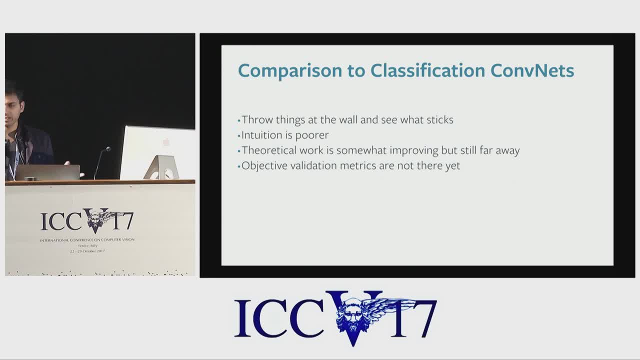 like loss, then GANs don't work as well. They're not very stable And why they work. the theoretical work surrounding GANs. we're trying to get there, Like many smart people are working on theories on stabilizing GANs, why GANs work and all of that. 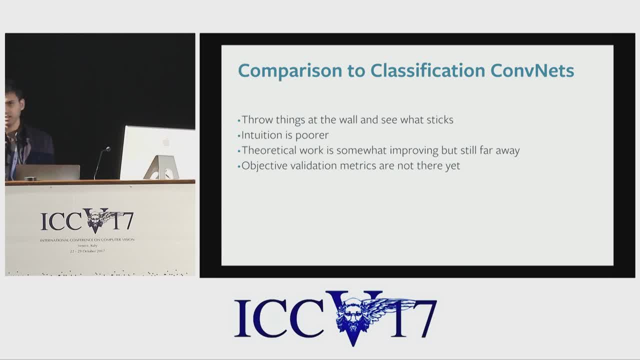 but still not there. And we're not there yet with objective validation metrics either, Like: how do you tell objectively Whether a GAN is working better or not? We have certain metrics formulated by the community, like inception score, but they're just not there yet. 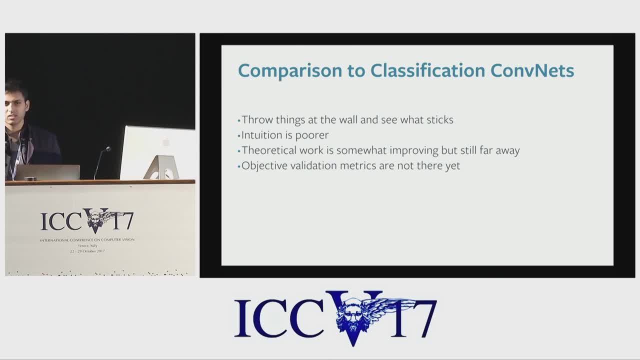 Like. depending on the data set and the scheme and the setting, these metrics are not as stable as some of the more traditional metrics you'd use in classification, for example. So, starting with the 16 tricks, I will tell you about how to train your GAN. 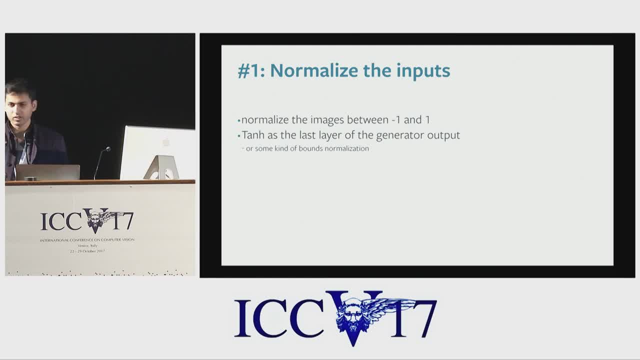 The first one is a very obvious one: Normalize your images to a particular range. The standard is like 0 mean minus 1 to 1 standard deviation. So if you do normalize your images, you would also want the last layer of your generator. 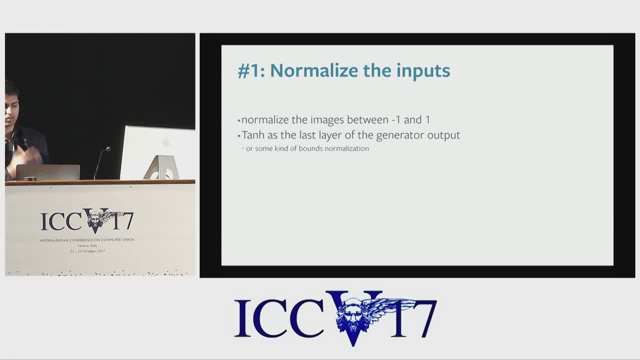 to have some kind of normalization layer. I particularly use 10H, because 10H gives an output between minus 1 and 1.. But you can do it. You can use some variant that's nicely differentiable And for classic GANs, by classic GANs. 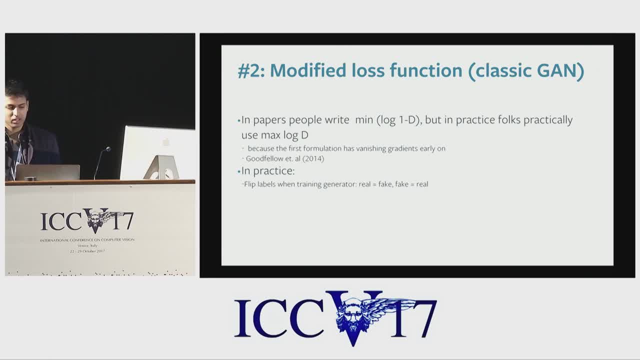 I mean in Goodfellow's original formulation. one of the small things we found was that practically people use the max of the log of the discriminator as the loss function rather than the minimum of log 1 minus d, And so we kind of change this up so that the map on the left 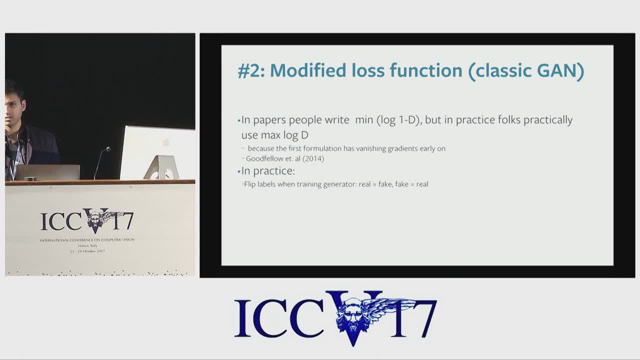 would be the lowest possible value on the left, rather than the minimum of log 2 minus d, And so we use 10H and we change the rate of the data in the GANs. So we could also do something with that. We could do a little bit of config and we could do some sort of stuff with that. So I will show you how to do this And really will show you how to do things. So let me get this real quick, So I will show you. I have a bunch of things that I can. 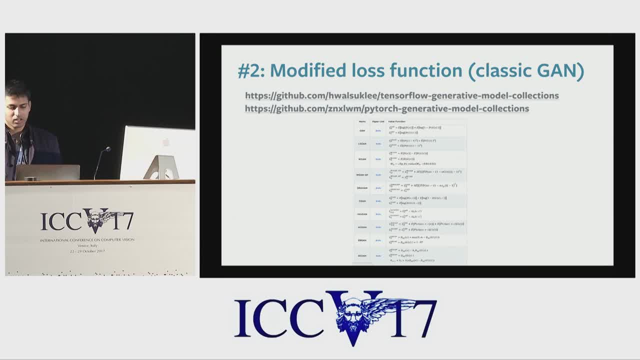 there's a lot of new loss formulations. there's this one table I found from from these implementations of GANs, where now they kind of show all the different kinds of formulations. I mean these are not even come like. this is not a complete list, but just over the last couple of years there's many different. 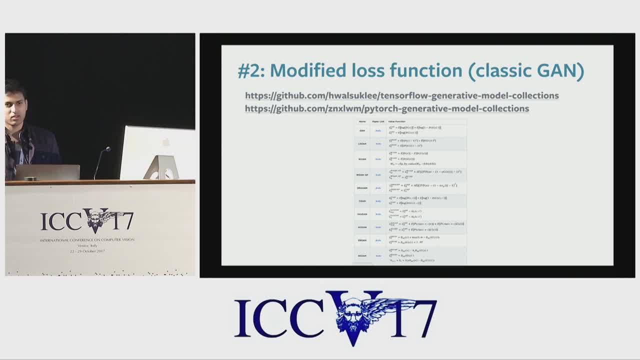 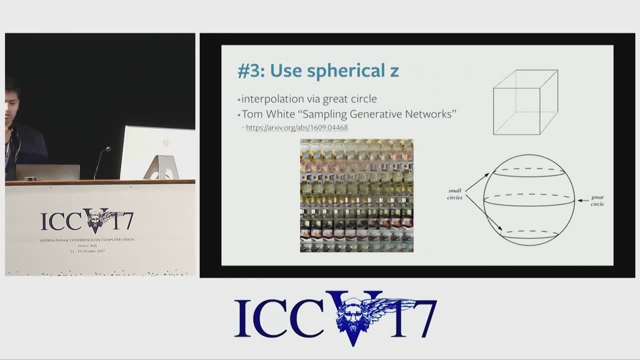 variants and formulations of various kinds that try to stabilize GANs in slightly different ways. one of the nice and important things to do if you want to do generations, if you want to do interpolations between generations, is make your noise be spherical so that you can go from one point to another. you can 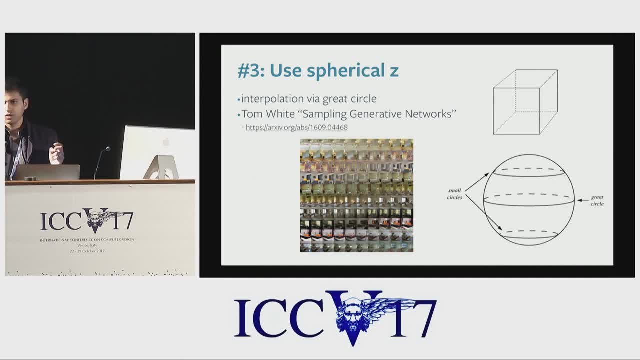 start sampling points with equal distance and if you are sample like if you're basically doing interpolations instead of going taking a straight line from point A to point B, actually go on the great circle, so sample points on the great circle and then give those points to your generator. 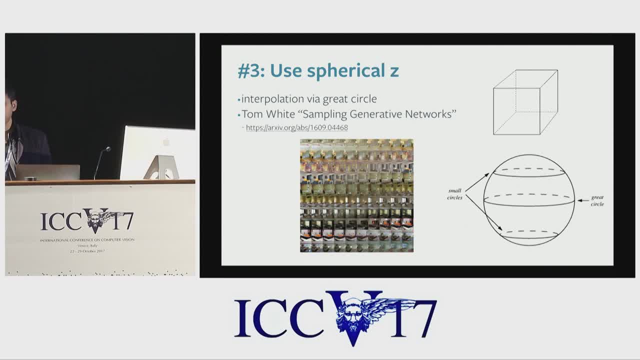 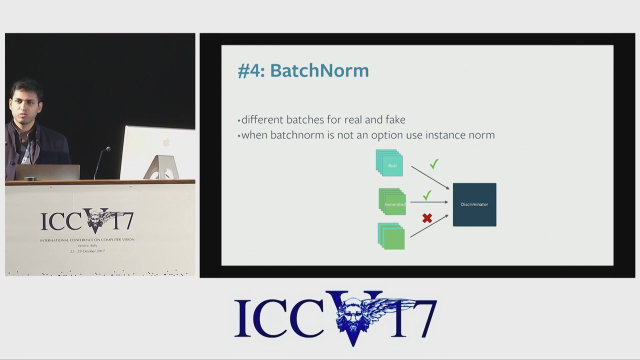 and the interpolations will be more uniform and smooth. and I'm waiting for slide 4 to appear. my computer is stuck, sorry. slide 4: batch norm. batch norm has been pretty useful in almost all of the GAN implementations I know, and there's there's several opinions on this, but one. 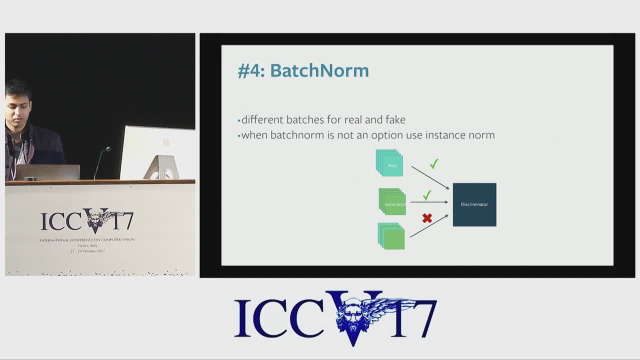 thing I found, and many of my collaborators found largely, is if because batch norm is so, because if you have a batch norm and you have a batch norm, if you have a batch norm and you have a batch norm and you have a batch norm, if you have a network that has batch norm, it's very dependent on like what. 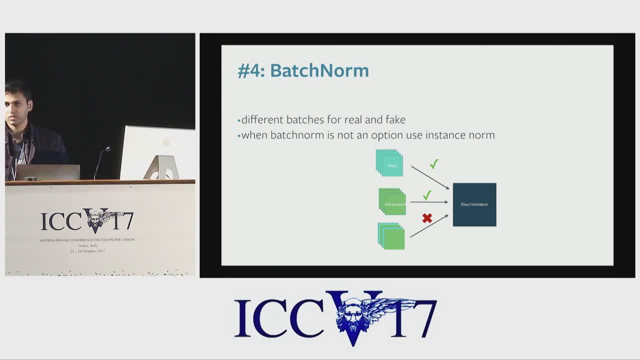 inputs you give your. your output is very dependent on that, so you'd want to give separate batches of real and separate batches of fake to your discriminator, so the discriminator could take in one whole batch of generated samples and then predict whether it's real or fake, and one and separately, one whole batch. 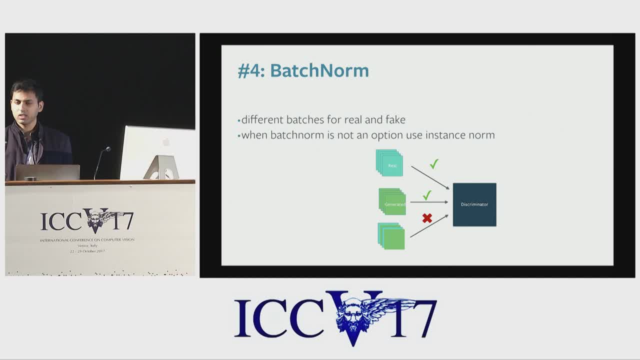 of real samples and then predict whether it's real or fake. but again, this is something that that I mentioned last time at- I think it was- iClear, and someone from the crowd came back to me and said: you can actually make mixed batches work. it's you just have to find different hyper parameters. 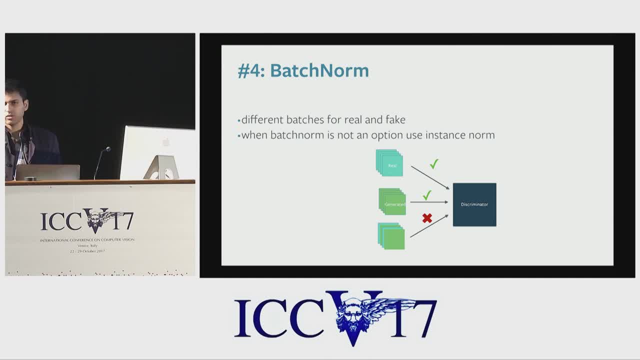 than the ones you would use for if you use separate batch of real fake. but practically this seems to work very well and I think it's very useful and I think it's worked pretty well to use different batches and in general, inserting batch norm in your discriminator especially seems to work really well, almost seems. 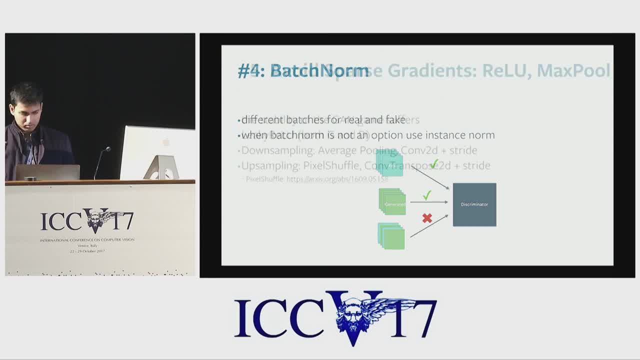 to be essential, okay. the fifth one is to avoid sparse gradients where you can. so if you have something like ReLU, you have zero gradients, for all of the activations in there are less than zero, and if you have something like Maxwell, you only have the gradient flowing through the max value and all of 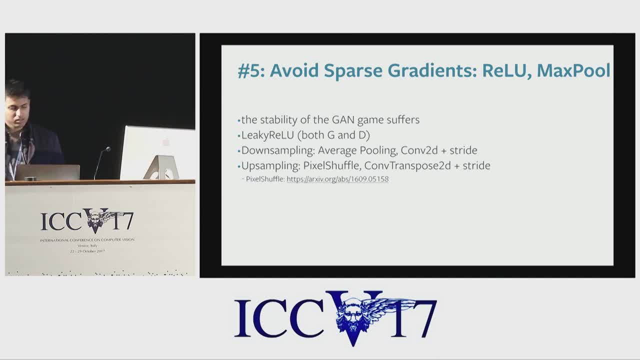 the other values in your window are zero. so generally avoiding these seems to help. in terms of architecture. search over many papers. we did find something like this. another thing is it seems to be pretty important in how you do up sampling and down sampling you. you have artifacts in. 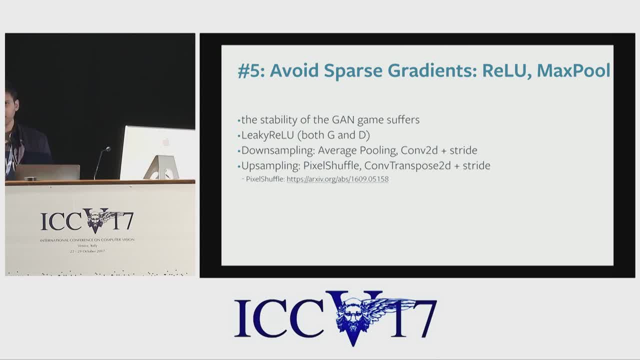 your generations that show up in many of the, in many of the pictures that people showed you today. there's these weird wavility artifacts that are showing up, and it seems that if you use slightly different up sampling methods, like pixel shuffle, for example, then you can get rid of these artifacts, and it seems to be this easy win that you 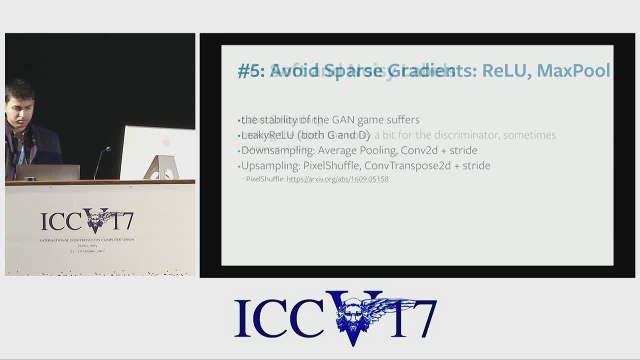 would get. and the sixth trick is, instead of using hard labels such as 0 and 1- for our like minus 1 and 1, whatever you use, use some kind of soft labels that the, instead of taking 1, it would try to do like a small 1 plus or minus. some noise. 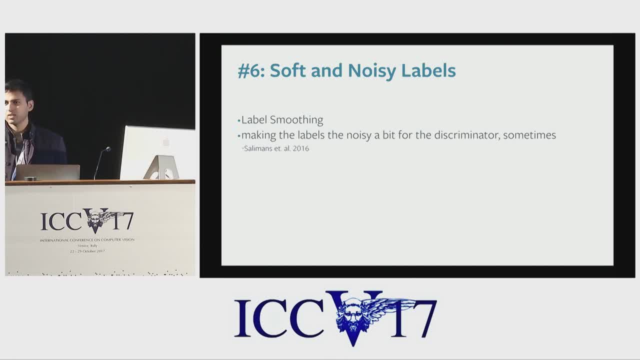 variable 0.9 sometimes, and like 1.1 sometimes and so on, and that seems to be helpful. it also sort of lines with avoiding making, just making the problem smoother, making the gradients sort of fuzzy. I don't know. it seems to intuitively make sense. but 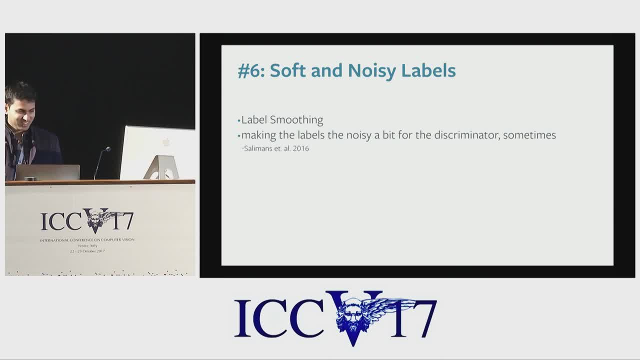 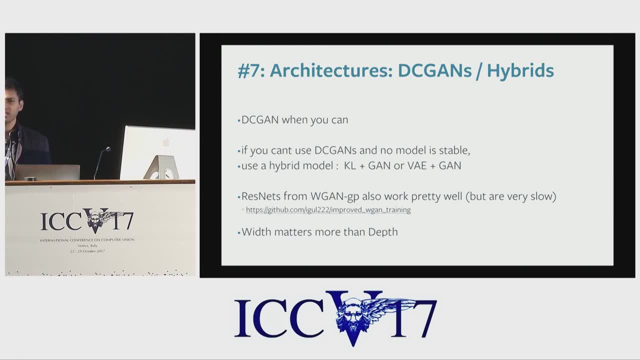 intuitions go so only so far. architectures: this is one of the important things. you take. you try to train again. you pick some architecture that's your favorite architecture and you try to use that in your GAN setting. it's likely going to fail. DC GAN seems to. 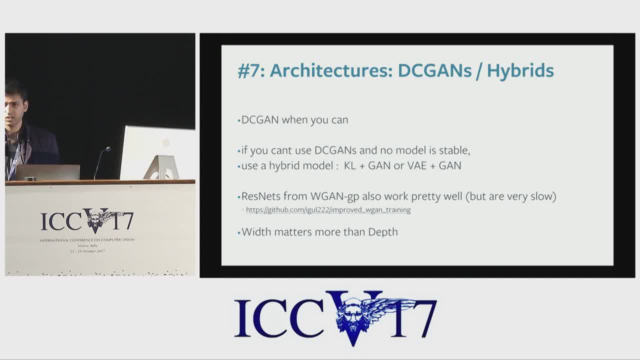 be pretty stable for all image generation tasks in general, especially like pure generations. if you have something like up sampling or picks the big style stuff, I think you can be more flexible in your picking your architectures. if you can't use DC GANs in general, it seems to help to use some. 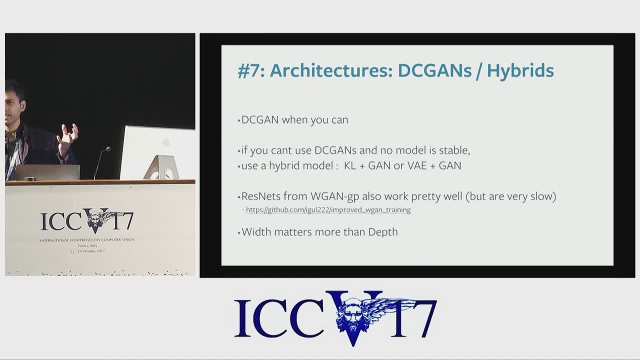 variant of loss where you have a GAN loss and some KL divergence like loss. Mihaela gave a talk about autoencoder GANs, which is kind of sort of in line with that suggestion, and the improved wasser stein GAN paper uses these particular. 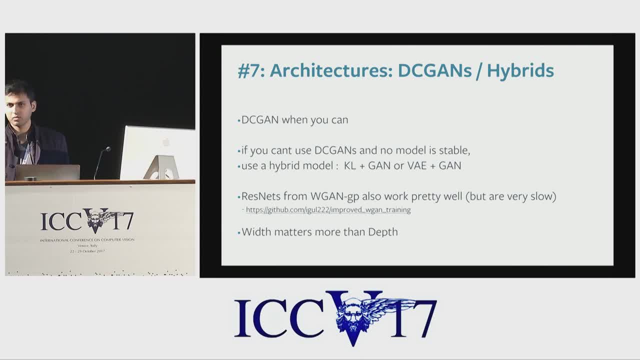 resumes and this seems they seem to work pretty well and almost all settings, except that they're really expensive to train. it might take like five times longer to train those. or say that a standard DC GAN architecture and one of the things that one of my collaborators is based off GAN discussion, in which I believe in terms of geb бcoughThere's supposed to be a specific application for a GAN mapping system. there's anгорthing for a GAN mapping for oldrutin or for algum brushes in your region. and while you're practice testing the data monitoring in the sobre elementary GAN permission, bulk-trying of GAN attached text file can support the sugar pointer at Iustere specifically and it's not implemented for improve long lasting research using Google. google they have to change sometimes it's guidelines for'. 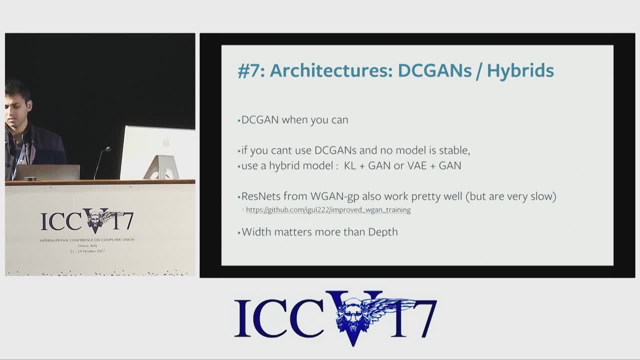 Martin Orjewski said is that as he's training these things, he noticed that width matters more than depth, Like if you find an architecture that's giving decent generations and you want to scale it up in some way, make your model wider. 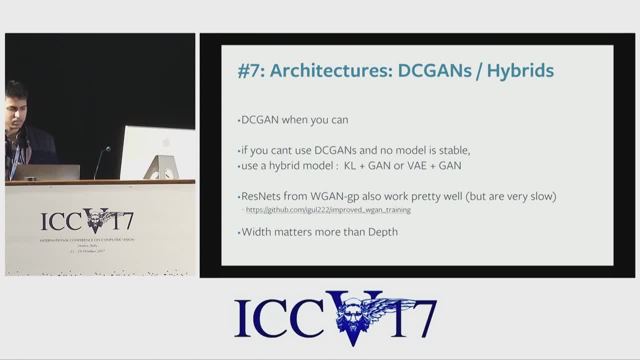 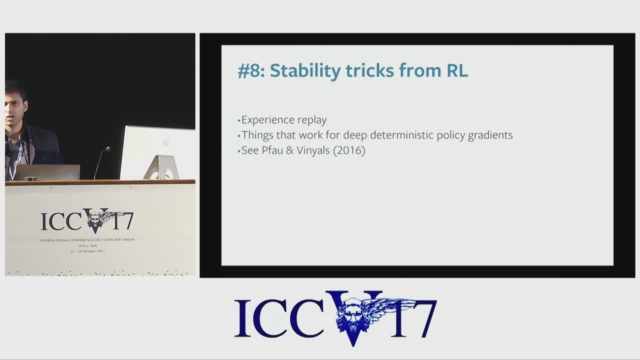 and it automatically seems to give some qualitative improvements. OK, OK. So the eighth one is: you can use tricks from reinforcement learning. So actor-critic models have a very deep connection to generative adversarial networks, And there's actually a talk by David Fa at 4.30 today on this. 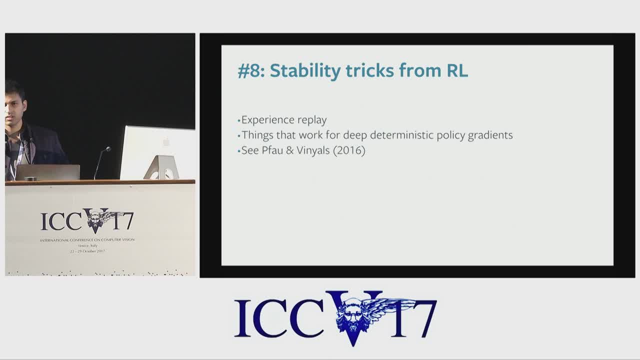 And so you can use things like experience replay So you can keep some generations from an epoch ago and regularize with those and do all of these things that you do with policy gradient methods. And the ninth trick, just a suggestion, is Atom as an optimizer seems to be working pretty well. 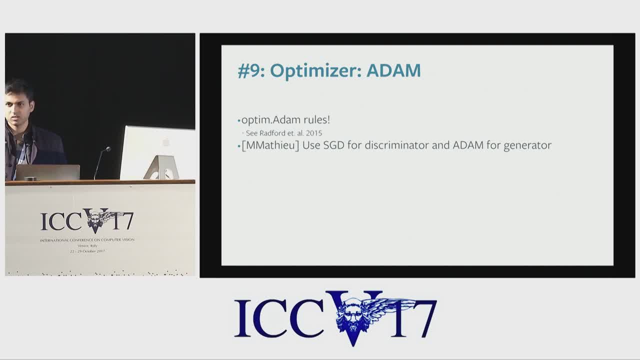 And almost all the implementations I've seen. just use Atom, Kind of works. could use that, OK, OK, OK, OK, OK, OK. And one of the things that Michael Matthew suggested- he's a graduate at NYU, he said- using SGD for the discriminator. 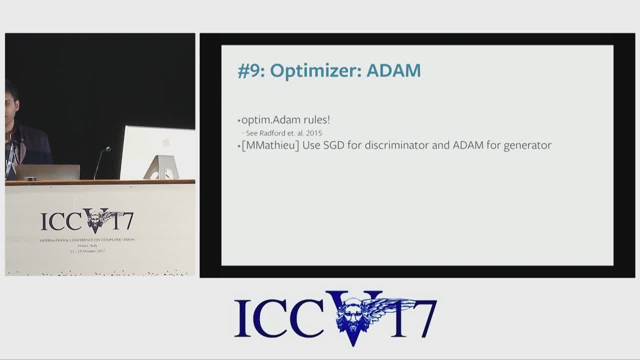 and Atom for the generator seems to work. He used to. he worked on video generation And he said it seems to work nicer. But I think that's a very specific suggestion Because Atom in general, everyone's been using it across the GAN community. 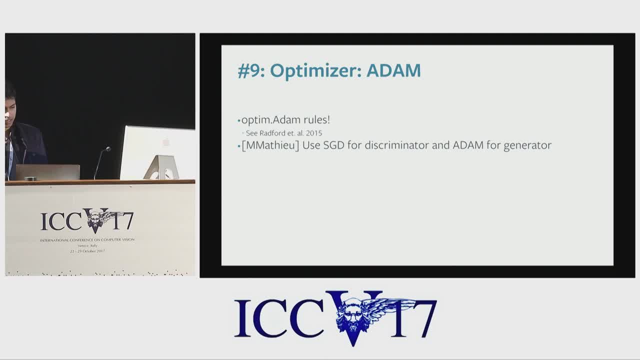 So feel free to start with that. And gradient penalty. So, with the introduction of the improved Wasserstein GANs paper by Ishan Gulrajani, and also with two other papers that have other motivations, one called DraGAN and the other one, 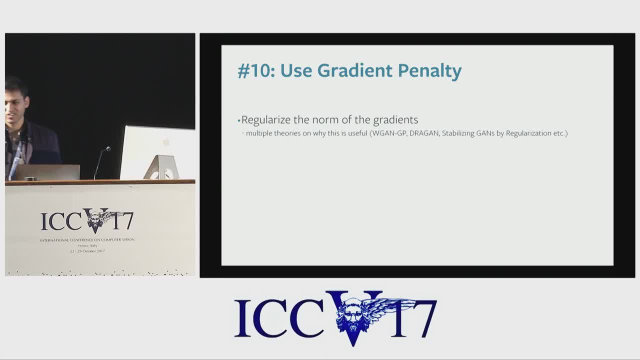 I don't actually know the full name of the paper is something like how to train a DraGAN or something like that. And there's another paper that comes to a similar conclusion, but from a regularization point of view, And they all seem to come to this conclusion. 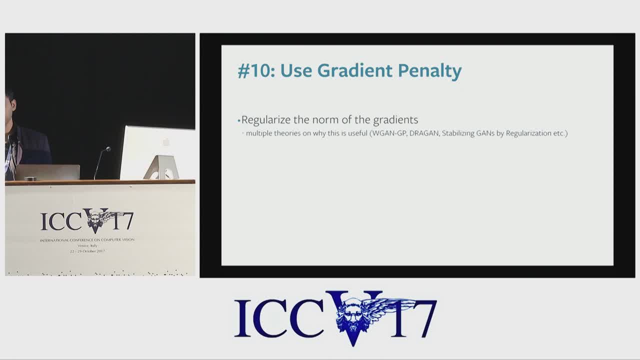 that if you can penalize the norm of your gradients, that is, you can take your gradients backprop through the gradient formulation itself where the norm is bounded, then that generally helps the stability of GANs And in practice it seems to be working pretty well. 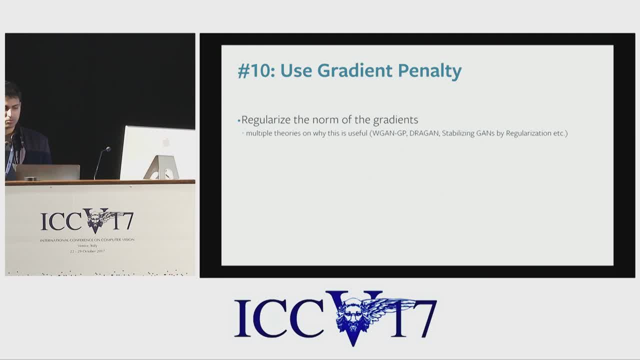 across many different settings. So that's one suggestion. It's kind of a little tricky to implement, but there's many implementations. There's many implementations. There's many applications of that in the most popular frameworks. It's tricky to implement by yourself because you actually 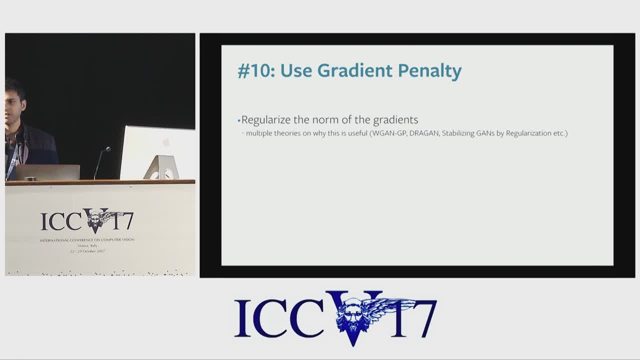 have to. your framework has to support taking the derivative with respect to the gradients, and not all frameworks do support this. So in 11, this is something that when I got into GAN research I was like: I mean not GAN research. 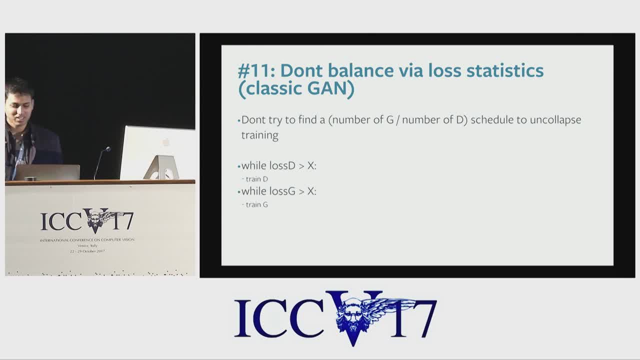 more like when I was playing with my scripts and trying to make them more stable. I was like, how do I make this training more stable? And one of the nice things you would want to try is: oh, let's see if I can create some complicated schedule where 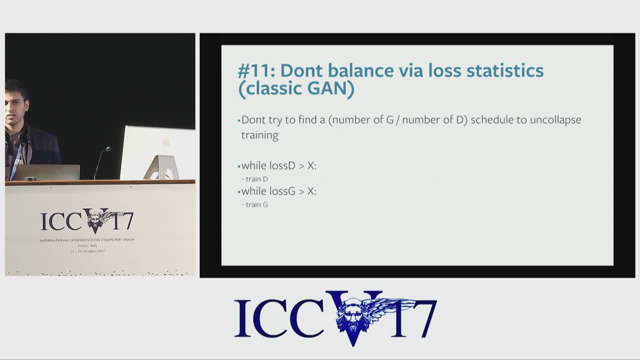 I can make the generator train for a little bit, and then I detect somehow that the discriminator is getting weaker And then I train that for a little bit more, and so on And finding such optimal schedules. I think many people across many labs. 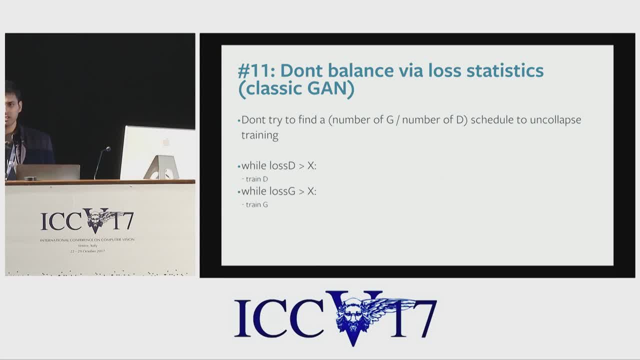 have tried to work on this And so far nothing has come about. So unless you have a more principled approach to this, I think just playing around with the code is unlikely going to help. 12th one is something that is a suggestion. 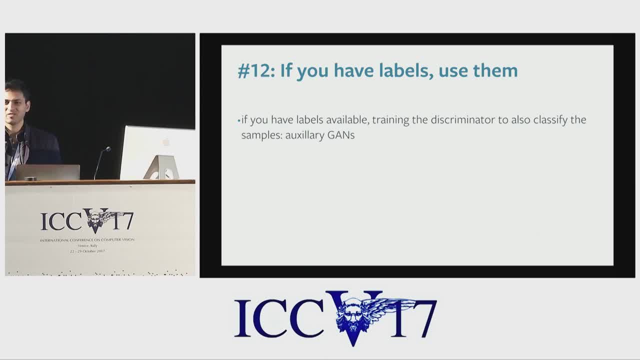 from across. all of machine learning is: if you have labels, use them. If you can do conditional generation for part of your data set, or if you can make your generator have some optionally- it can take labels or something. yeah, use the labels. 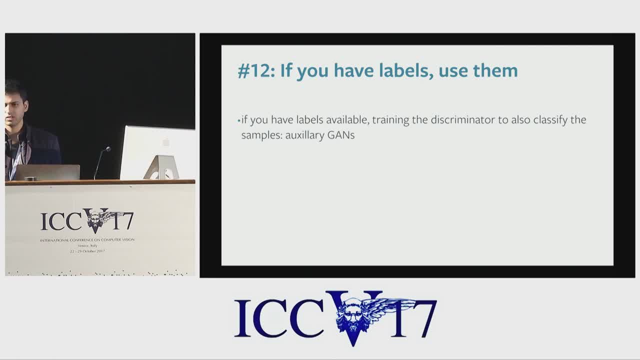 You can see this in the best ImageNet generations, for example. Yeah Yeah, Because you can use labels, use some form of supervision, And this is true from across many different problems for video prediction and generating cipher images and stuff, The conditional generation seems to always help. 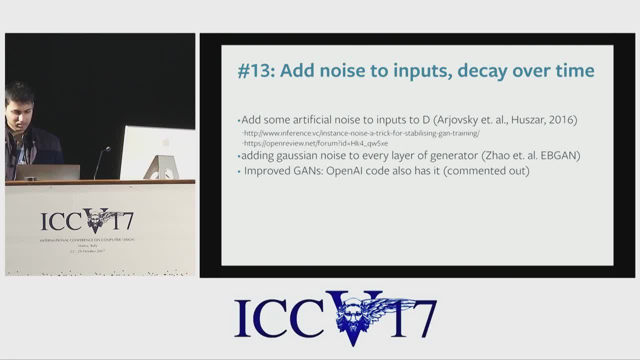 This is is something that I think It still applies, but probably largely complementary to the norm of the gradient stuff. You could just add noise to the inputs- the real inputs- so that the discriminator's problem is harder. It can pick up on some artifacts in the real versus generated images and then just try to discriminate between them. 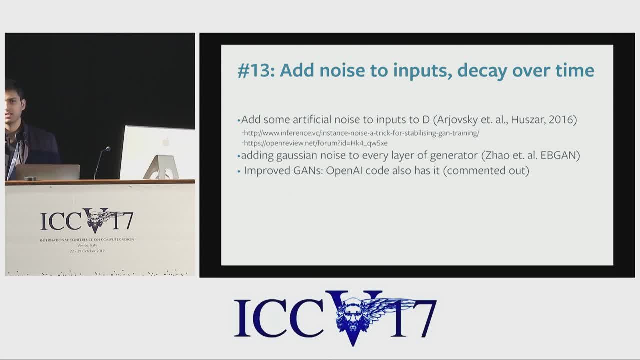 So it's just a trick that's saying, okay, let's make the discriminator's problem artificially hard And even if the generator sucks, then this will be regularized initially in training by doing this. add noise to inputs trick. Okay, So one of the things that 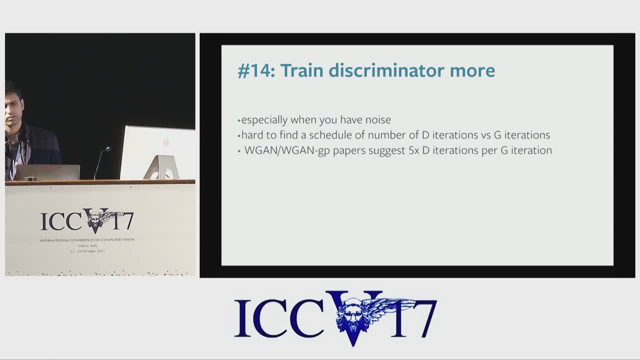 One of the things that was empirically suggested before things like Wasserstein GAN came out, but seemed to be supported by some theory, is that if you can train the discriminator more, in the Wasserstein GAN- or improved Wasserstein GAN- papers they suggest that you train the discriminator five times as well. 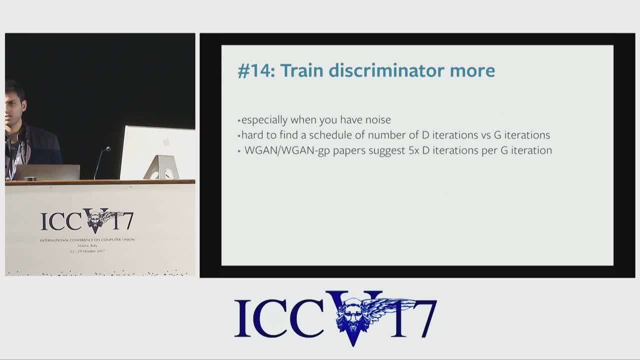 Yeah, So like if you can train the discriminator as much as the generator, or like try to train the discriminator until the discriminator loss goes to zero, and so on, this is something you could try, but in practice it's like, then your experiment takes like five times longer or something more. 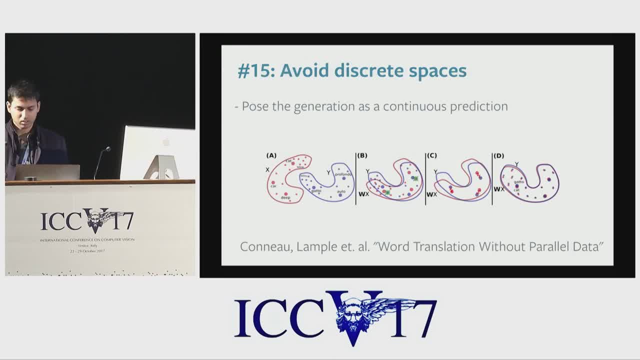 So one of the things: if you look at all of the people trying to apply GAN to text, you would find that it's really hard. Yeah, It's hard, It's hard, Yeah, Yeah, Yeah, Yeah Yeah. 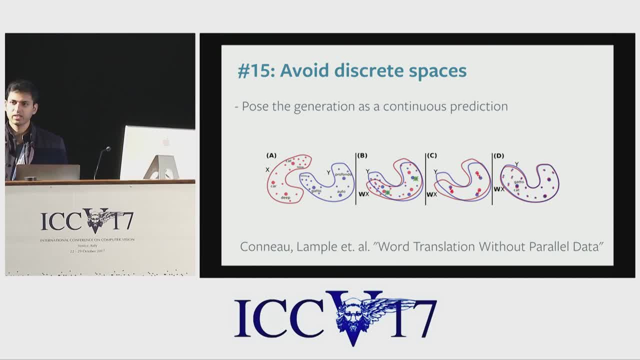 Yeah, Yeah, find that doing GANs with discrete spaces is pretty hard And one of the recent papers that just came out from my colleagues, instead it does GANs on text. It does these language-to-language word translation. So in the whole pipeline, the GAN part. 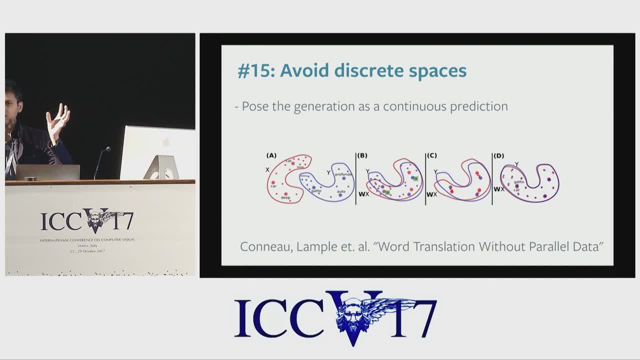 it just reposes it as predicting a rotation matrix from one manifold to another And now it's become a continuous prediction task. I've read other papers in the text setting that try to directly make the GAN generate word embeddings in other language and stuff. 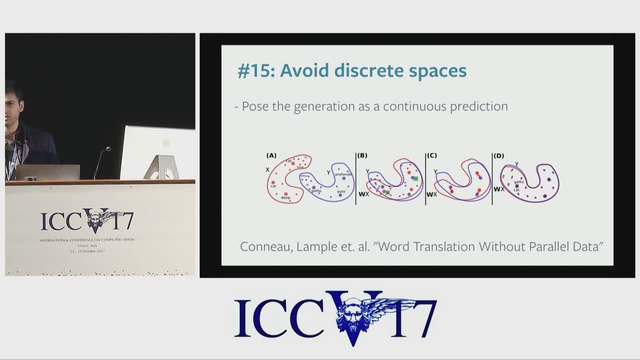 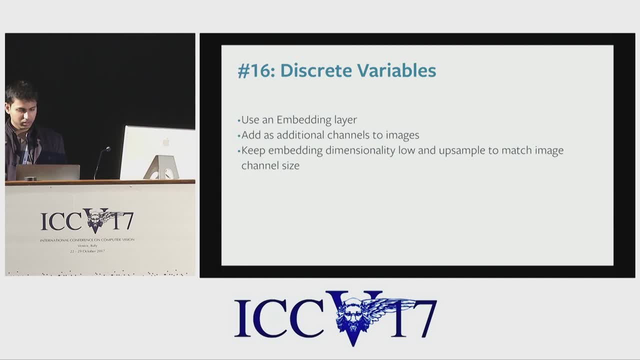 And that seems to be harder to get working in general. And one last trick: it's about conditional GANs. This comes from Emily, Thank you, She's from Canton at NYU. She says: if you want to do conditional GANs, 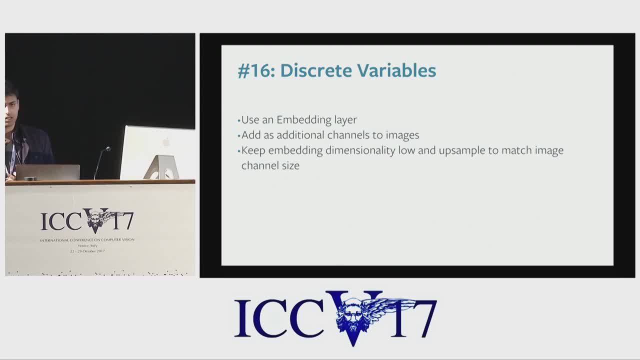 let's say you want to do text-to-image or something like that and your condition variables are discrete, then add some embedding layer where from your discrete condition variables, like from your one-hot encoding for discrete variable, you could go through an embedding layer. 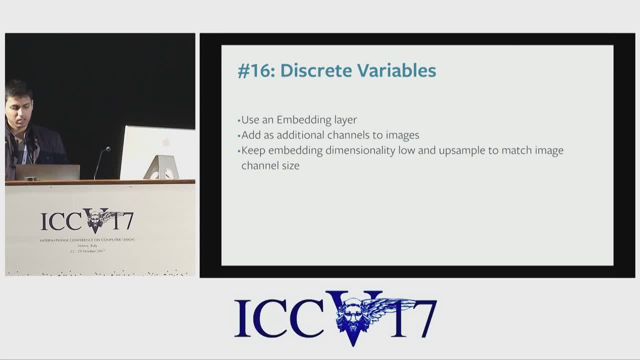 get some embeddings that you learn over the training And you can add these as additional channels to your images or your initial nice variables. That's pretty much all I have. The theory of GANs is improving overall thanks to the work of very smart people. 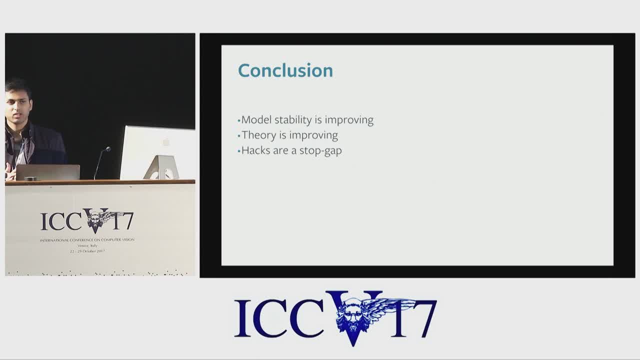 But in the meanwhile you kind of need all these hacks to get going. Thank you, I think I have 45 seconds. 45 seconds for a question, OK, I don't see any hands up, so no questions. Oh, there is a hand up. 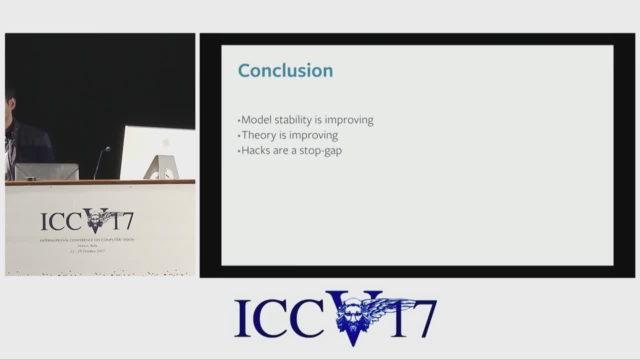 So how would you exactly define that the training is stable? How do you define that training is stable? Is it testing your patience? Maybe that's kind of like I don't know. This is the problem with GANs: You don't even know how to quantify whether training 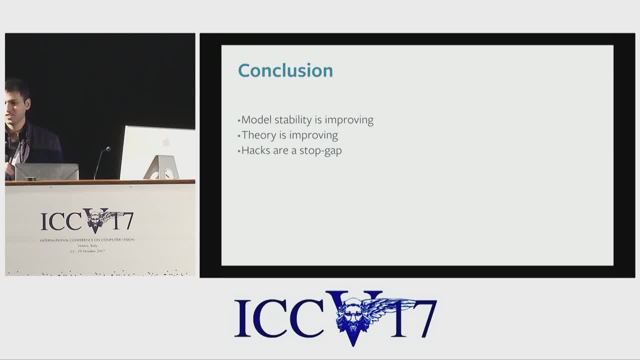 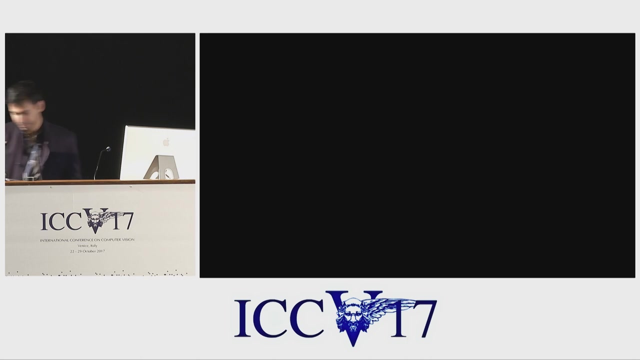 is stable or not properly. One way is you can just train over multiple hyperparameters and see if, on average, the training is stable with this inception score or something like that. But these are not yet properly formulated by the community. Thanks, Thank you. Thank you very much. 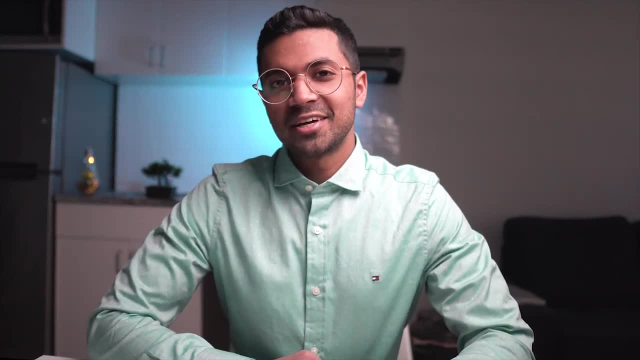 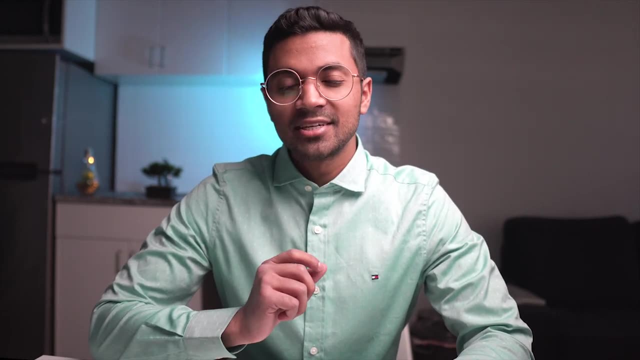 Hey friends, my name is Osama. Thanks for joining me. Today I'll be discussing one of the most fascinating nuclear reactor designs, which is the CANDU. It's one of the world's most safest and innovative reactor designs and it's truly a Canadian legacy. In this video, step by step: 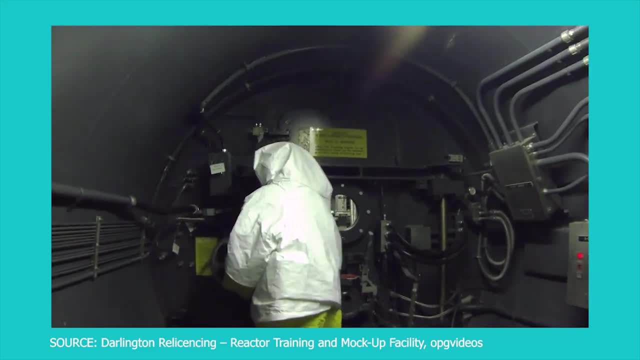 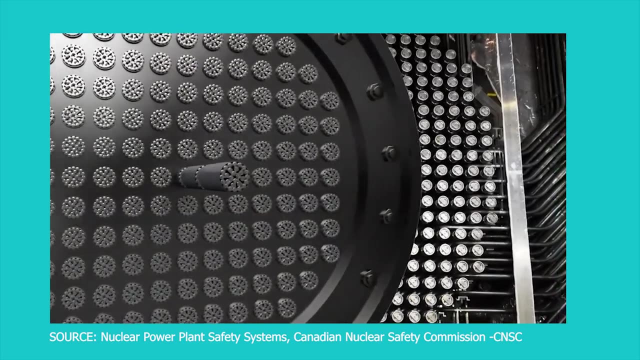 I'll be breaking down and simplifying the heart of the nuclear reactor. I'll start from the outside and slowly work inside. Think of this like a phone review, but for a nuclear reactor. So let's get started Now. what is the CANDU? The can in the CANDU C-A-N stands for Canadian, because of its 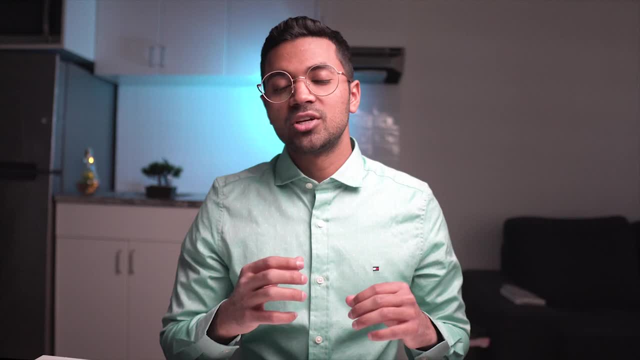 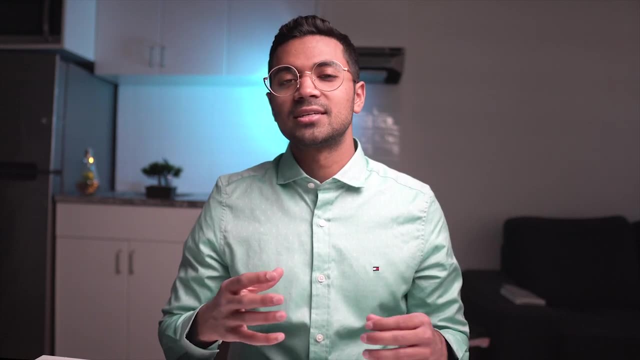 Canadian heritage. The D stands for deuterium, which is another word for heavy water. It's a unique attribute in this reactor. It's what makes it different from some of the other reactor designs that use light water instead of heavy water as a coolant and moderator. And three is 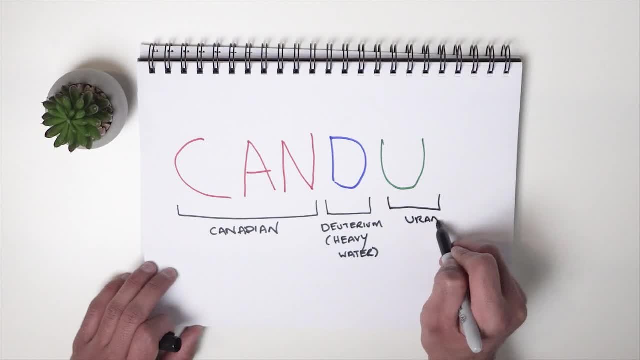 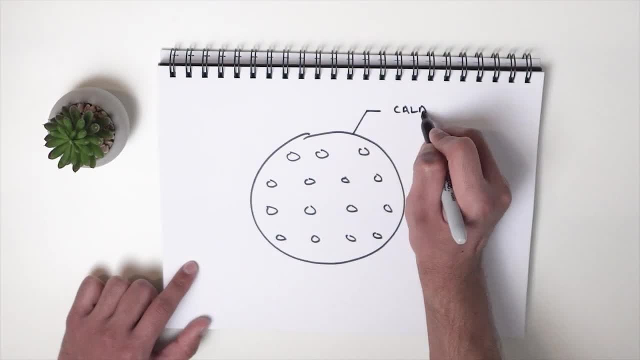 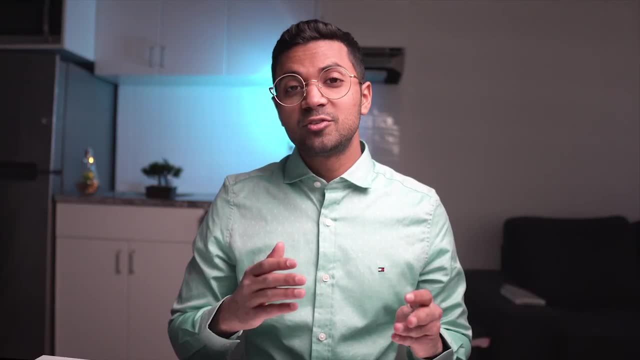